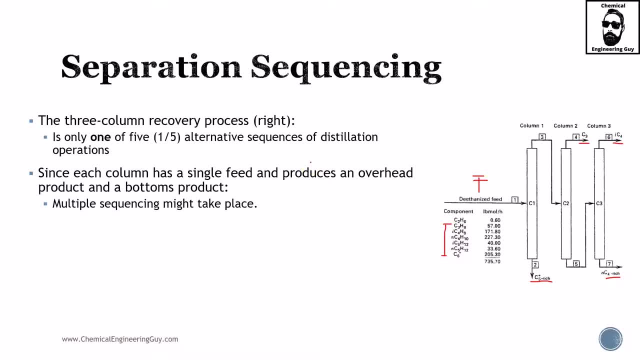 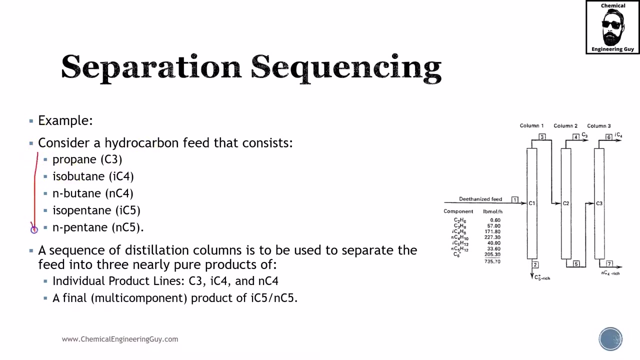 separation. sequencing is, of course, understanding the general rules for separation and what is the main focus? first, obtaining purity, maybe second, uh, energy requirements and so on. okay, so small summary, or to take from here is: multiple sequencing might take place. So we got the hydrocarbon feed, remember C3, all the way to C5, maybe even C6 and heavier. 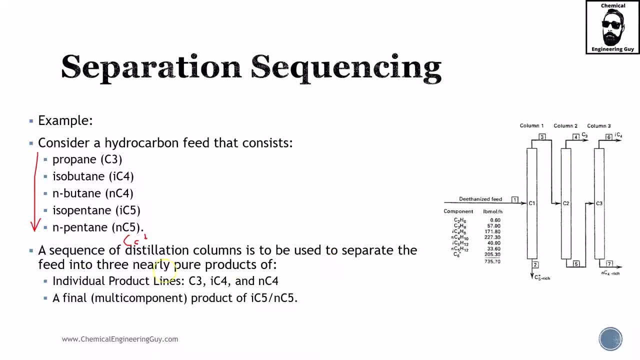 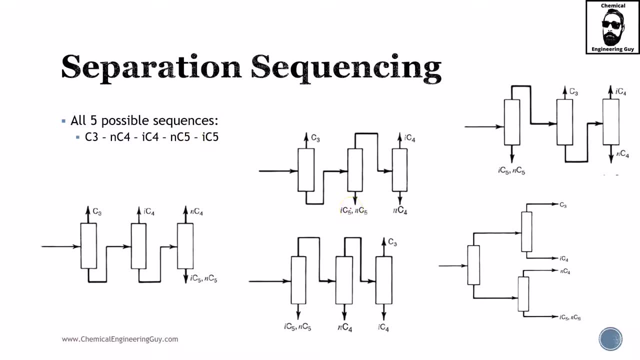 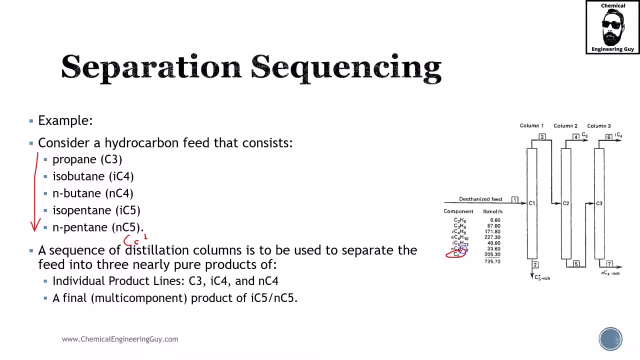 A sequence of distillation columns to be used, as stated before, And what I want to show you here, guys, is that actually we can have a lot of other separation schemes and unfortunately, okay, the following diagram contains nC5 and iso C5, meaning that We no longer have this guy right here. C6, but you get the idea. 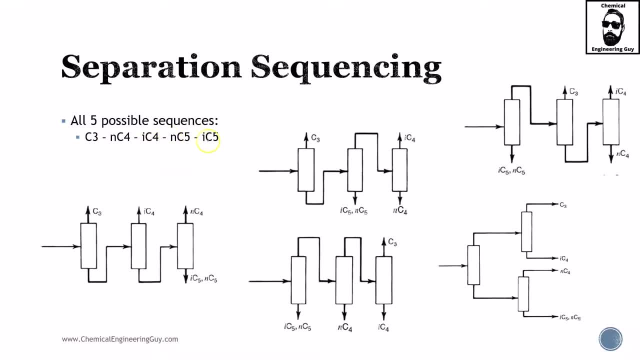 So we got C3, 4, 4,, 5, 5.. So this is normal ESO. remember, normal is this shape. ESO will be this shape. For n, pentane will be something like this. For ESO, pentane will be something like this: 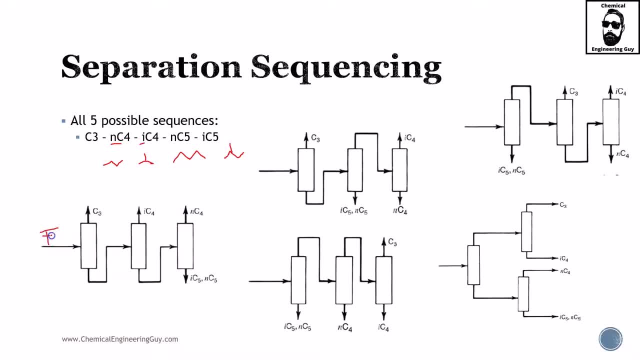 Okay, So what we are doing here is: we got fit and these are just arrangements in how we call a theory. separate them. It doesn't mean necessarily that this can happen, but these are approaches in which we are going to reach the streams as stated. 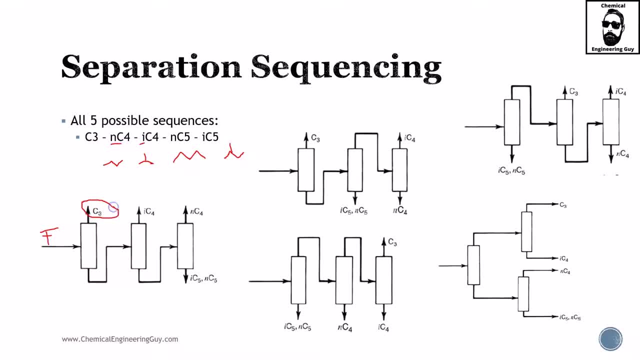 So the very first approach will be, of course, go for propane, which in theory is the lightest one. So we separate the lightest material and the heavier material, which is C4s and C5s, treat them later. So what you do is now remove the second lightest, which is ESO, and then n-butanes. 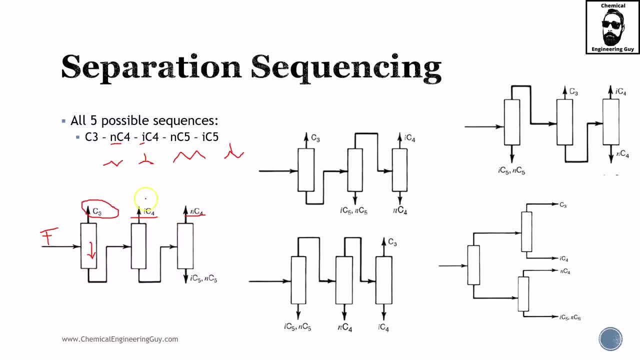 So I'm not going to get into technical terms. Okay, Chemistry, but typically ESO materials are easier to separate due to their Van der Waal interaction being not so strong. That's one approach. Maybe we can go as stated before, we separate C3, but in this specific 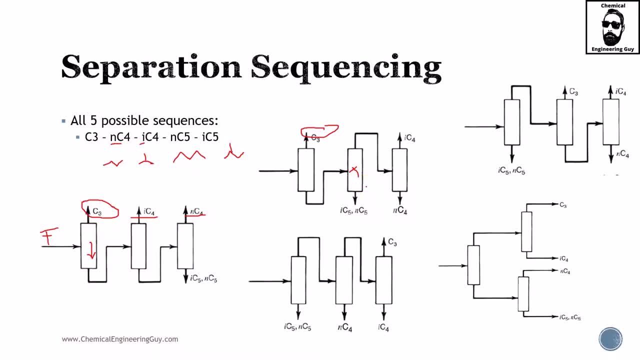 case we can separate half and half, So we separate C5s and we separate C4s and then we purify C4s. That will be a cool approach. The other one will be: Separate the rough heavy material, C5, and recover C4, C3 on the bottoms. 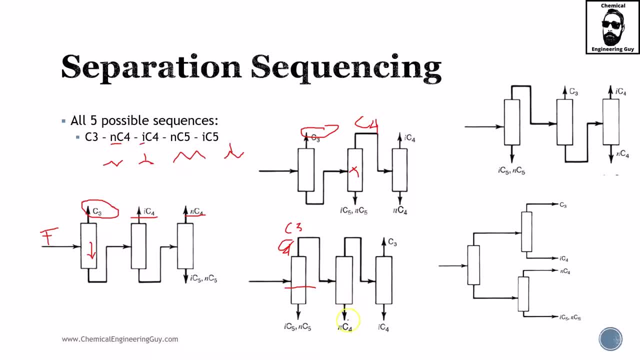 also in the distillates. send them to a second column, separate normal C4. Remember that ESO C4 and C3 are lighter. So we have C3 and ESO C4 and then separate. Another case which is also very, let's say, computing or mathematical: 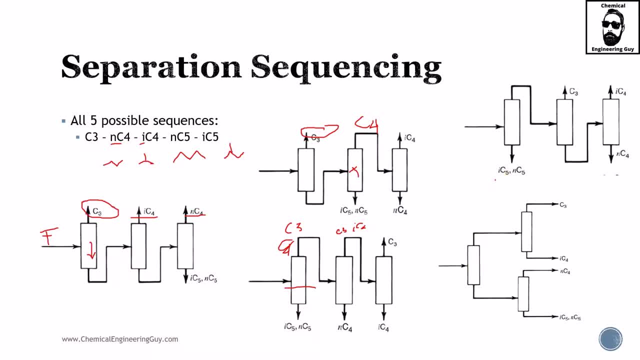 This is actually the one I always envision in my head, because remember that distillation columns are nothing more than trays. So I imagine having this tray system and saying: well, why not go half on half? So we got C3 all the way to C5.. 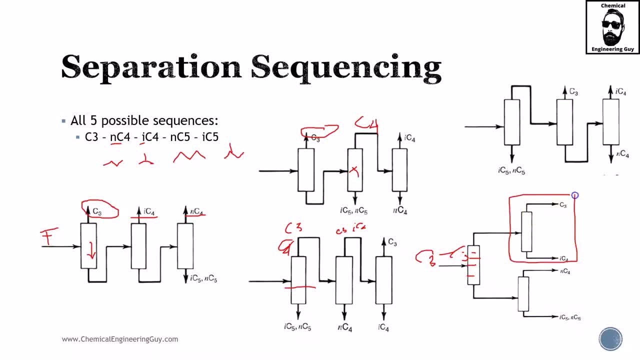 What we are doing here is top materials will be the most volatile material and the two materials going here, those will be the least volatile materials, And then I will separate them into the most volatile material, least volatile material. And so you keep doing this. 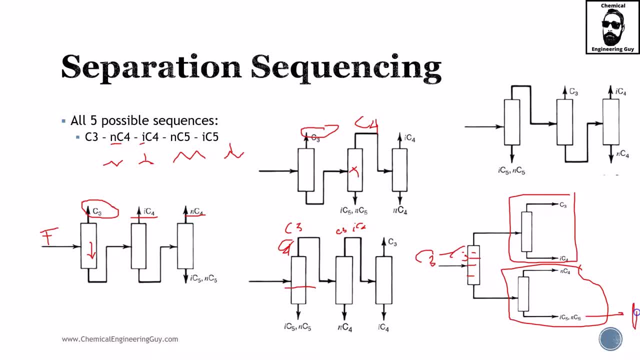 So actually, if you wanted to treat this one, you could do the same, but right now we're not focusing our attention into separating uh dependents, So this is my first approach Whenever I imagine some distillation column is separating roughly half and half. 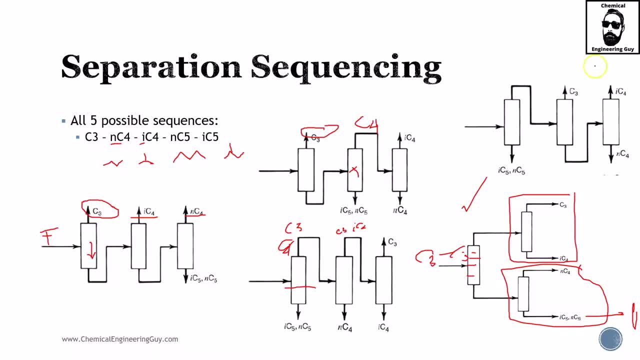 and with half by half, by having, and so on, And finally this one, guys, but there's no case of analyzing this, The main idea you got it. There are many ways in which we call, in theory, have a separation, actually depending on the sequences we're going to. 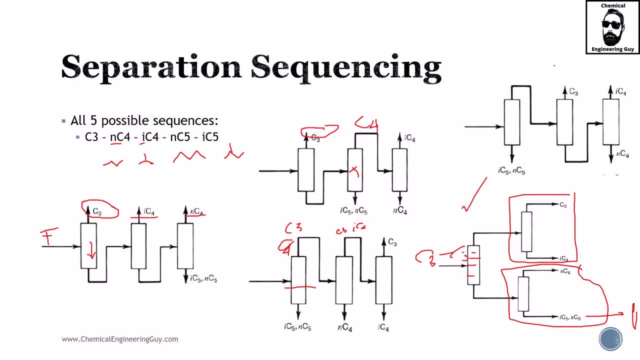 encounter that in some cases we favor certain properties or characteristics, For instance purity. in our cases we might favor total flow rates. In other cases we may favor, uh, the heating and cooling savings, and so on. There are many ways and many things to analyze. 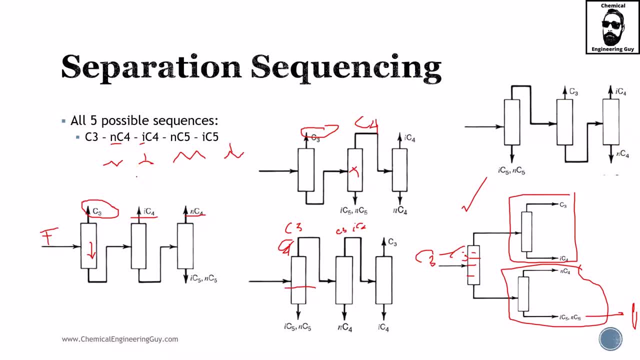 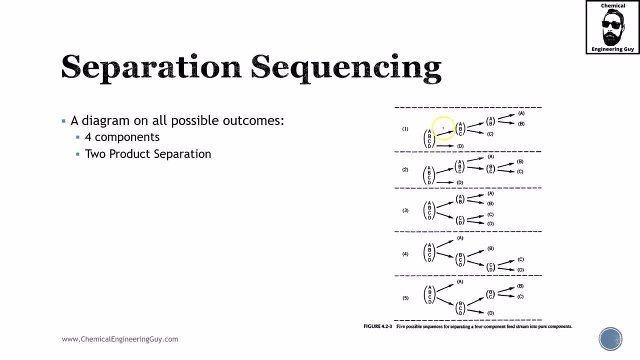 I cannot show you directly which one is the best. Of course we have some heuristics and thumb roads which we are going to be covering Next. Okay, And this is another diagram, how we can separate AB and CD. So the first one will be separate D, then ABC, then separate C. 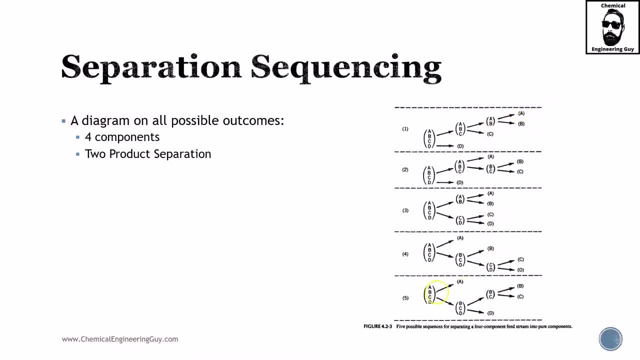 Then we have AB and then separate AB, or the reverse: We separate the lighter one, always the lighter one heavier, And so on. There are many ways in which we can separate. this. Actually, as stated before, is one of my most common approach. 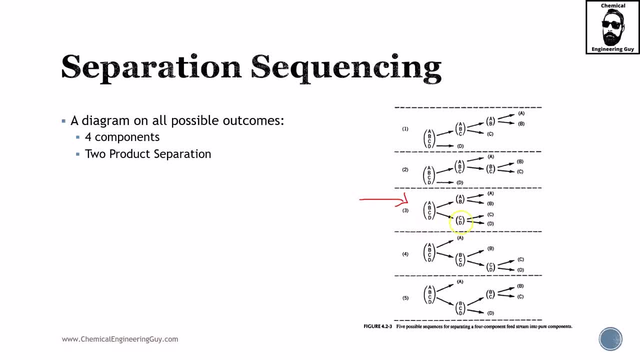 Whenever I see separation is separating half and half AB and CD, and then AB and CD are separated into halves A, B, and then C and D. 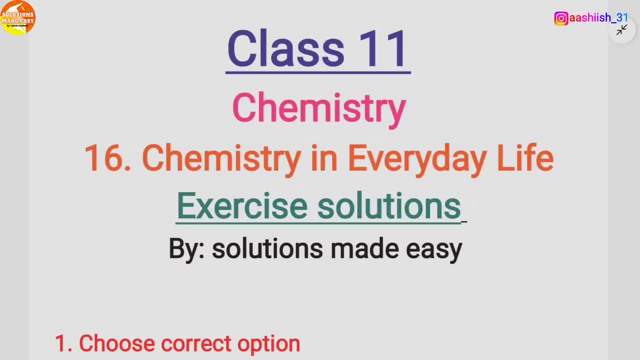 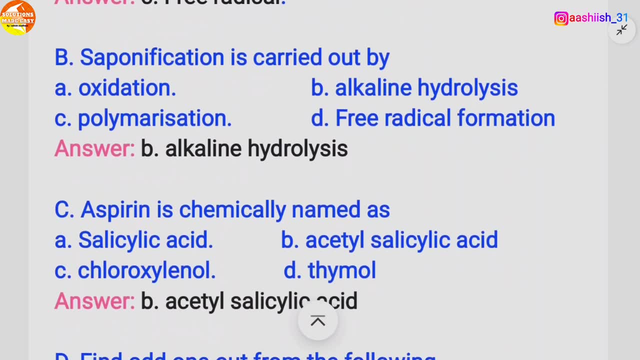 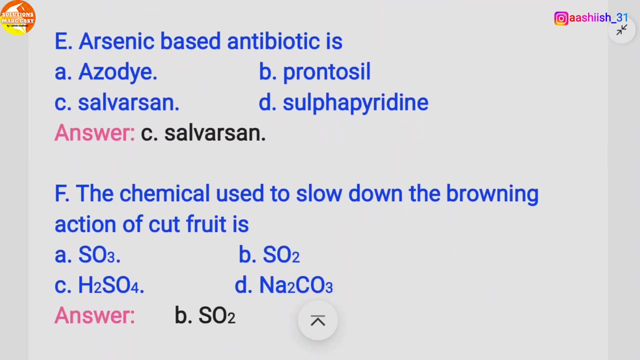 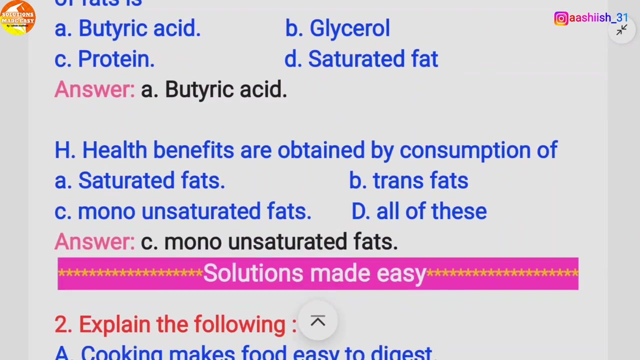 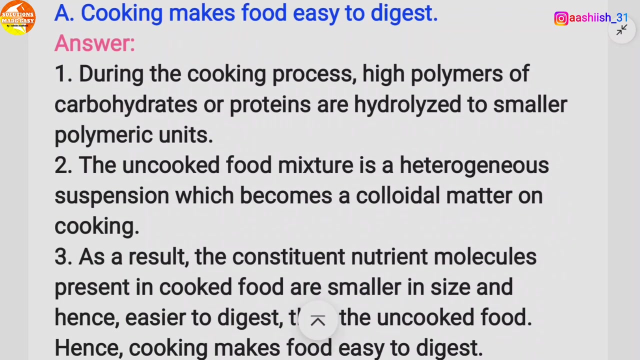 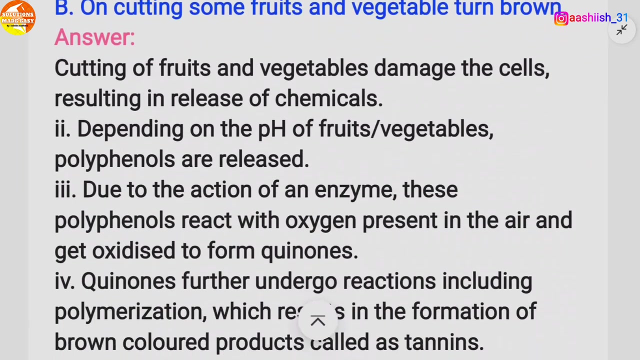 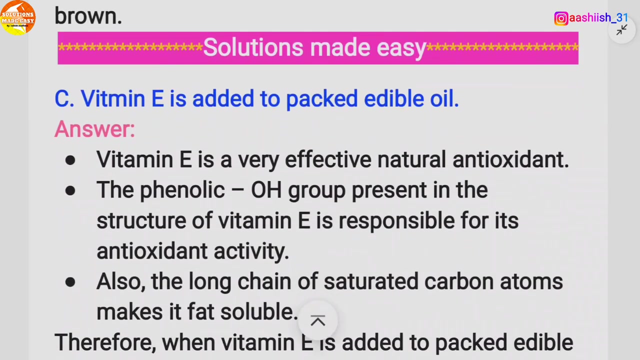 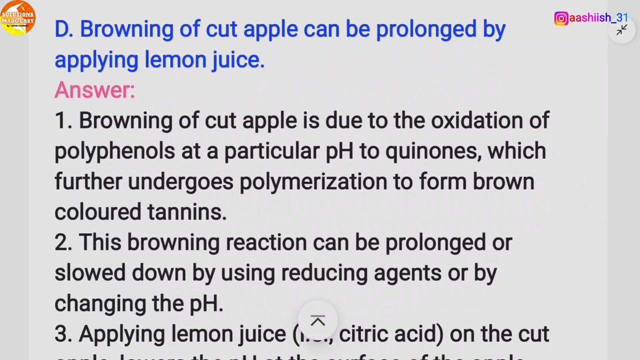 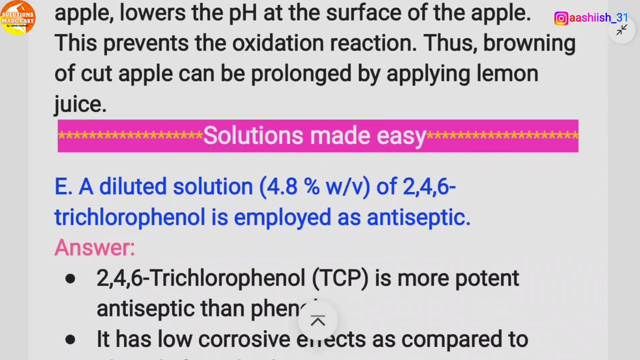 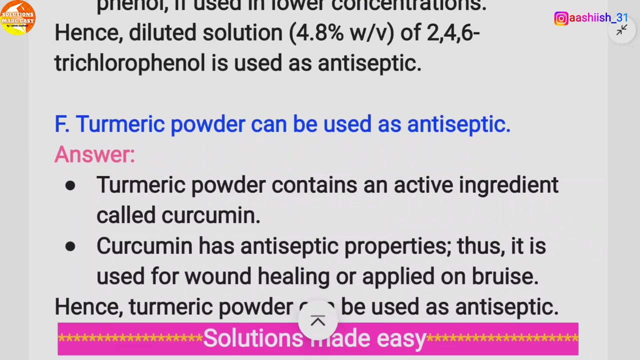 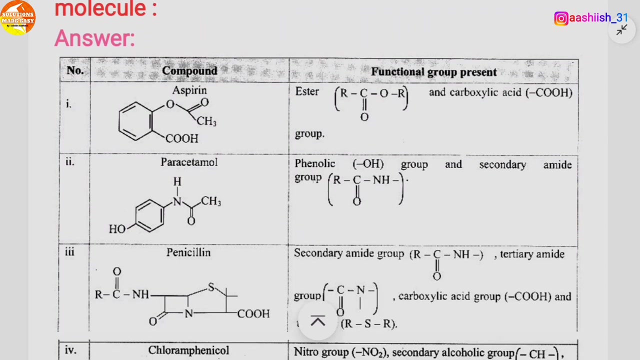 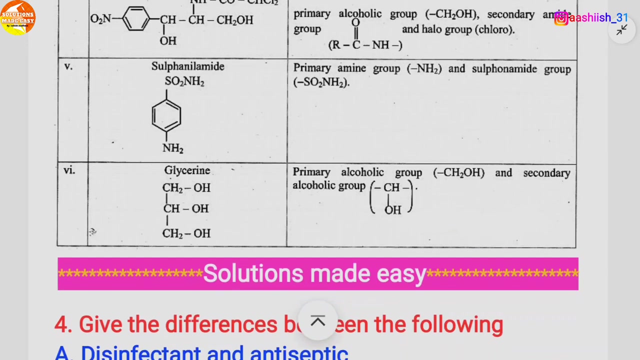 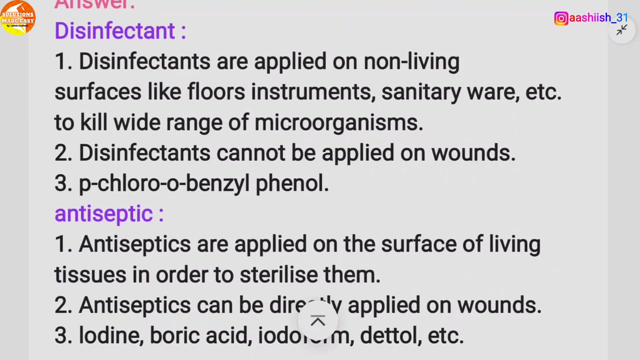 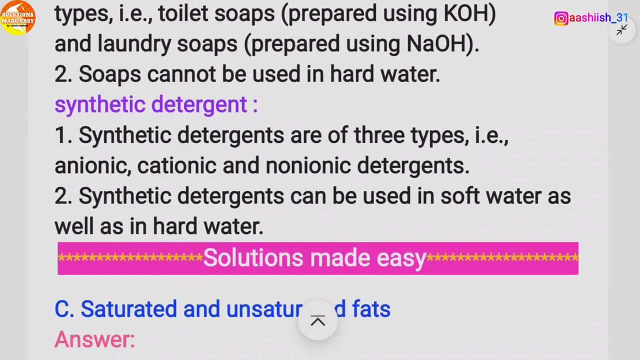 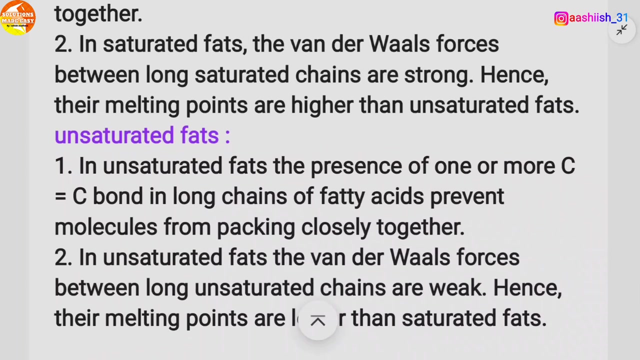 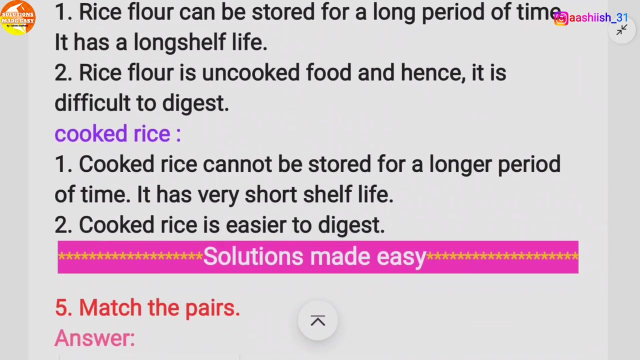 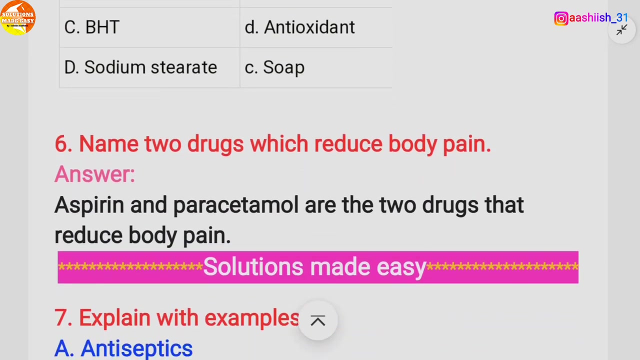 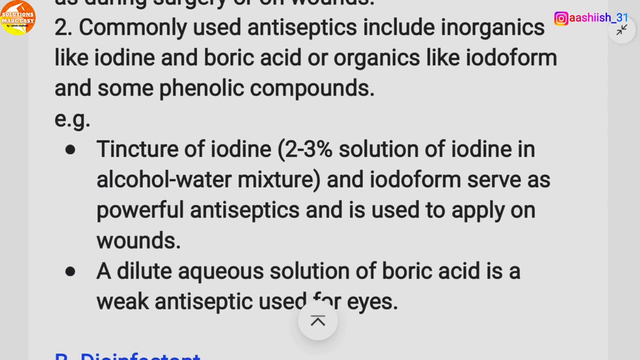 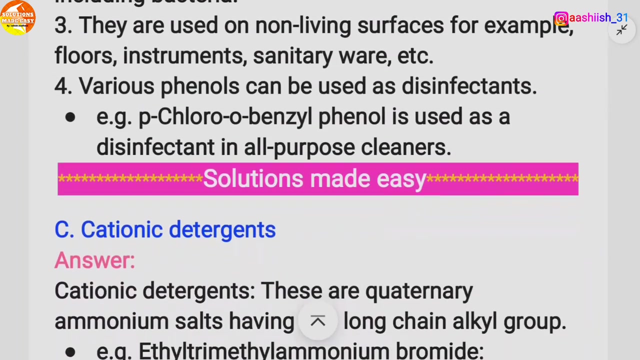 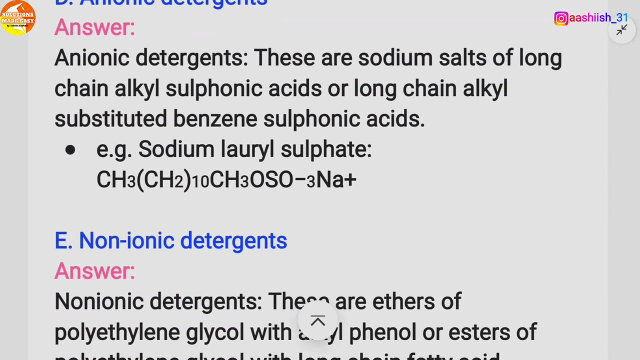 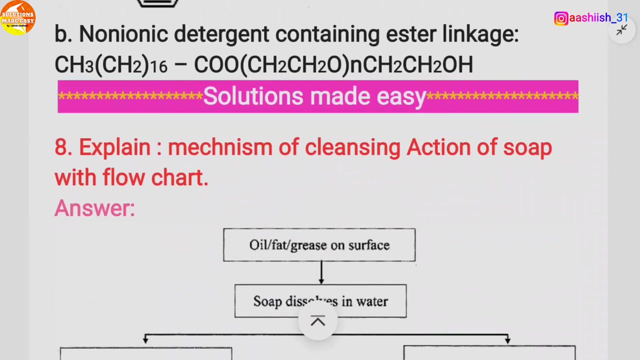 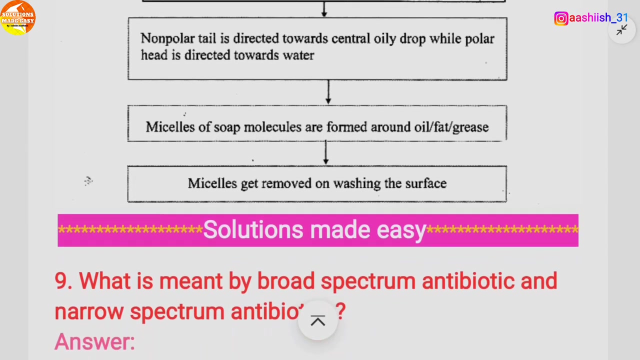 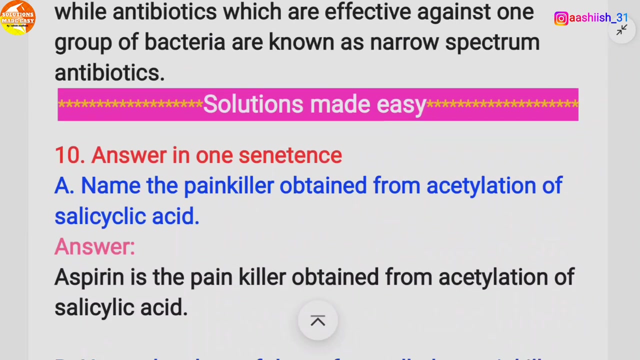 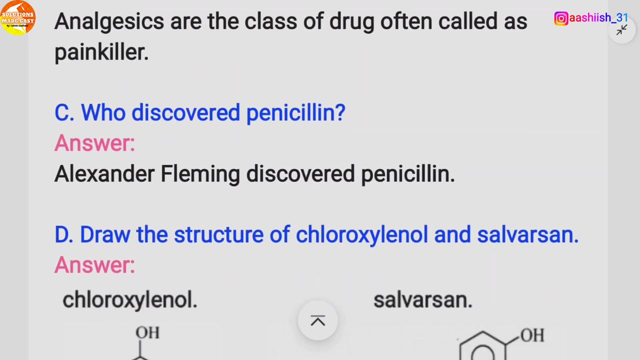 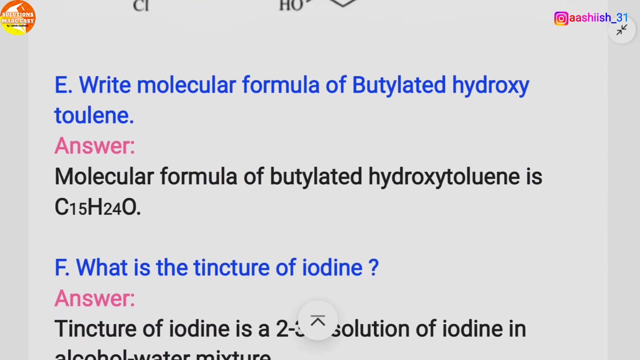 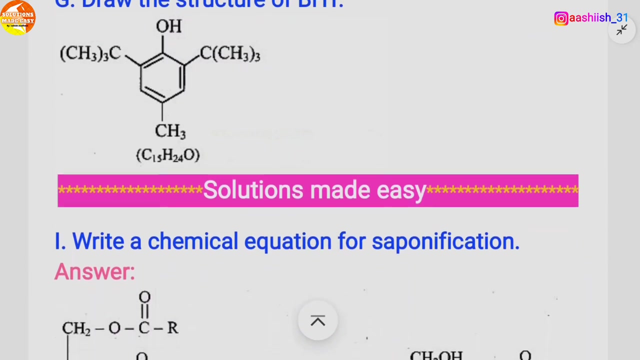